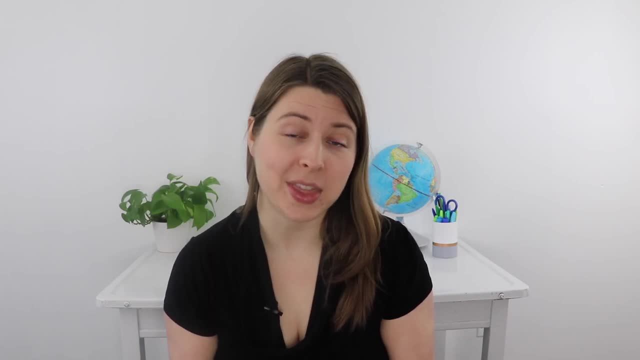 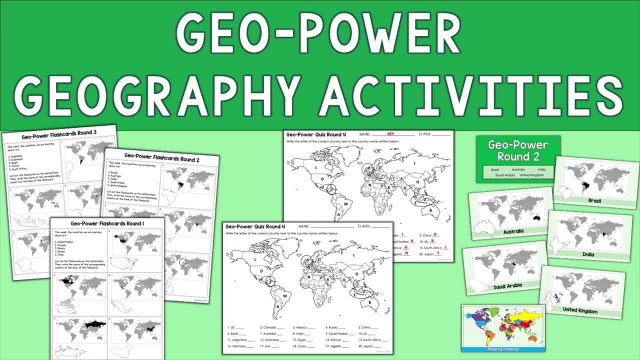 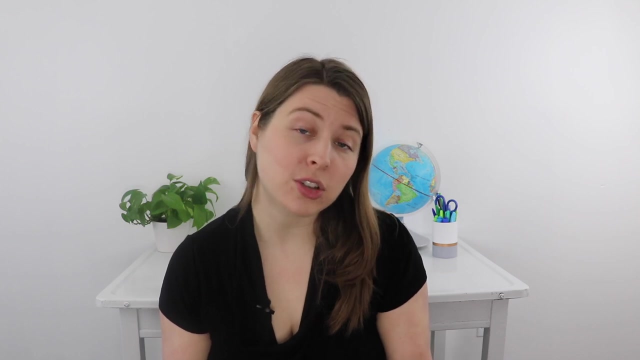 and so i'm thrilled to share that. i created the system that i call geopower, and this system breaks down different geographical locations, depending on the version that you're using, and students learn it over a sustained period of time, and it continues building on each other while also still 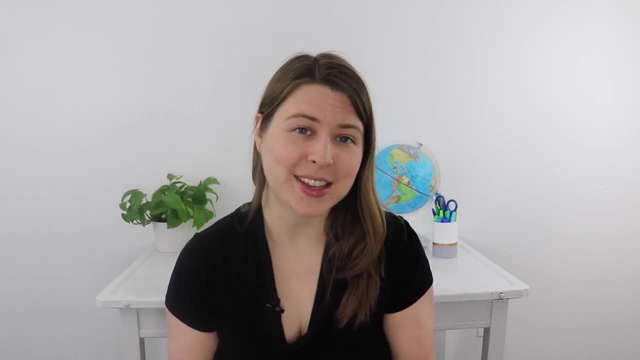 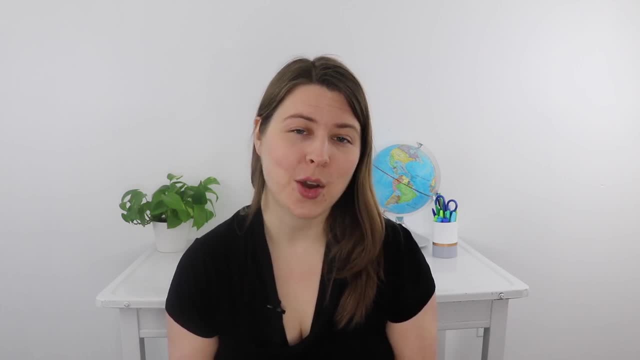 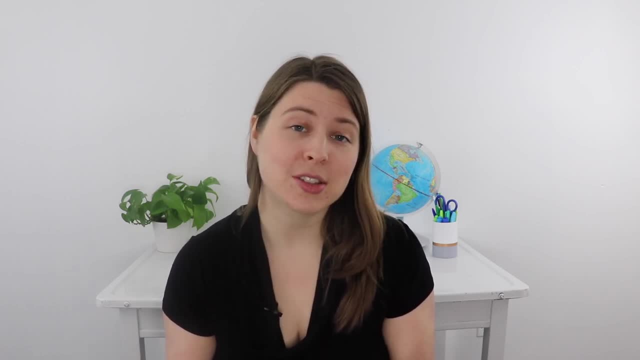 the students for three grade levels went through it. the students could still identify the 80 countries that we worked through over the past year, even though it had been over nine months since we had talked about any of it. that works, so i'm thrilled to share this and, like i mentioned, 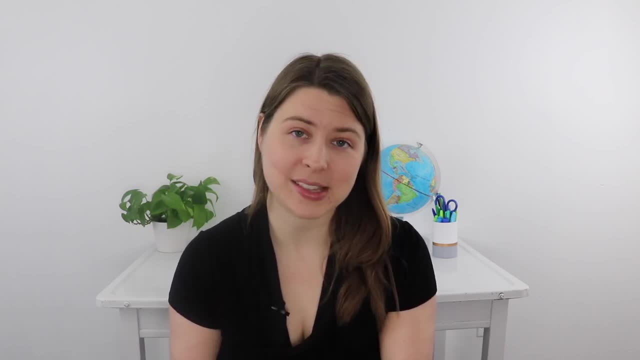 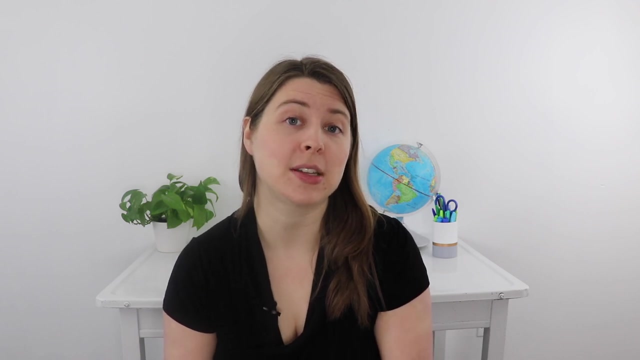 have expanded the program and i want to walk you through how to do this today. of course, you can totally create this yourself. that's what i did and, believe me, it was a labor of love, a very time consuming process, or, if you want this pre-made printable and ready to go and implement immediately. 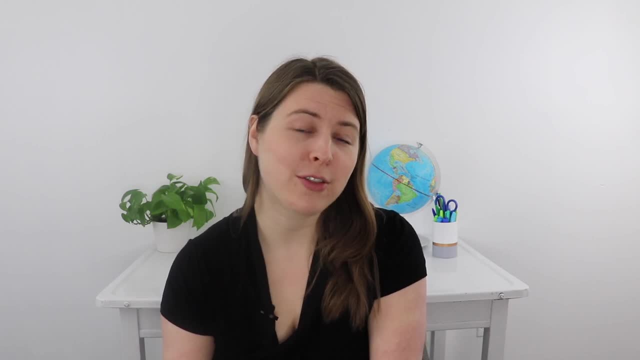 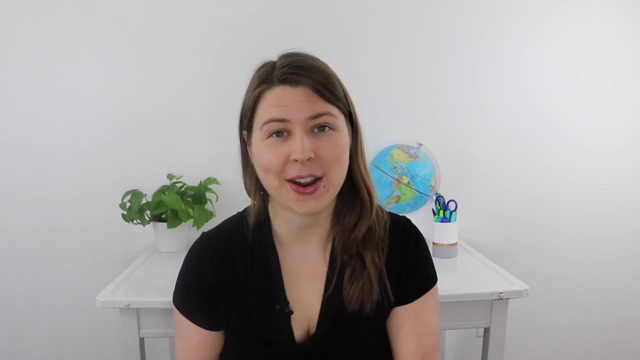 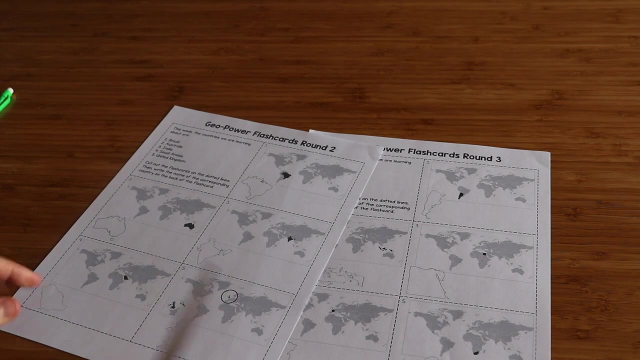 i will include links below and actually, as a special, i'm offering 20 off any of these bundles for the next two weeks, so starting when this is uploaded, until mid-february. let's break down how this actually works. first, you pass out flash cards to your students and the set of flash cards only. 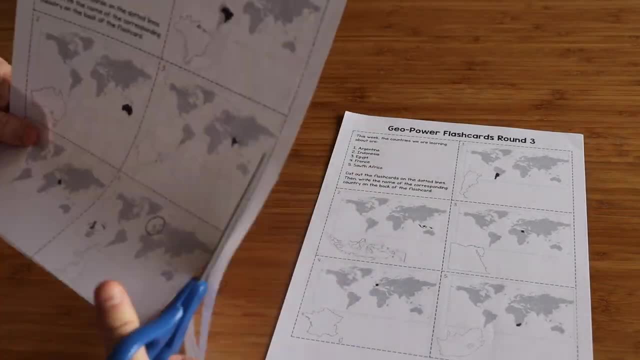 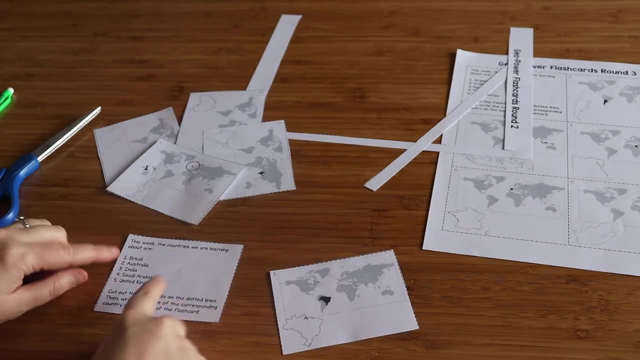 contains five countries. you don't want to do too much because it becomes overwhelming. students cut out the flash cards and write the name of the country on the back of the card. now they have a really simple study tool they can use to continue learning about these places as well. 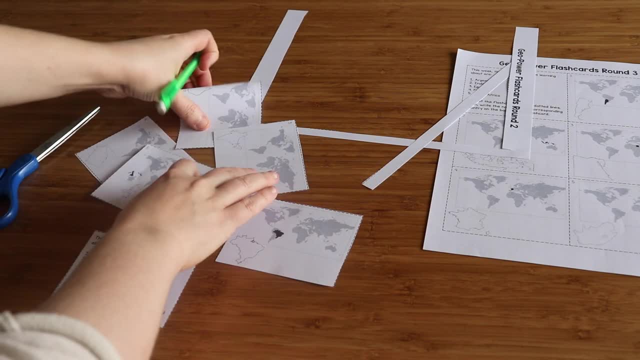 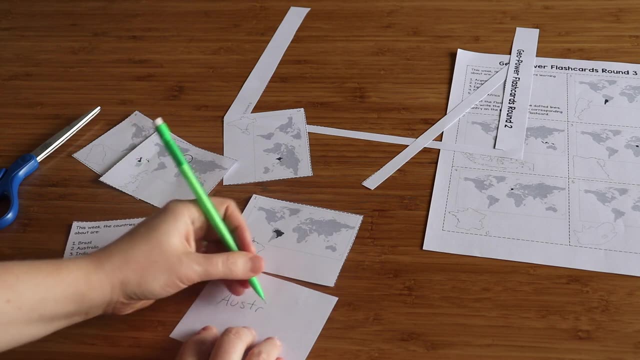 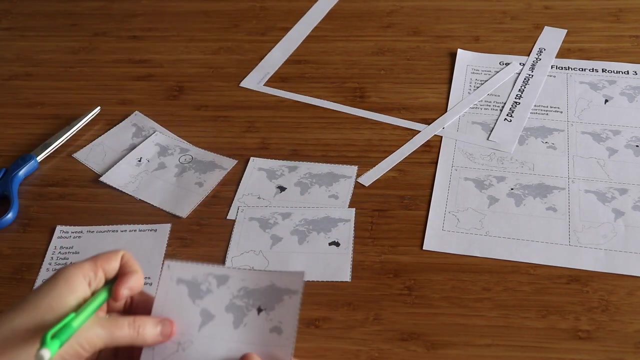 as continue reviewing and to make it easy, on each map there is both the country outline itself as well as a larger world map where you can see exactly where that country is located. So it's a perfect mix for both. It's also a great chance to talk about some of the cultural elements. 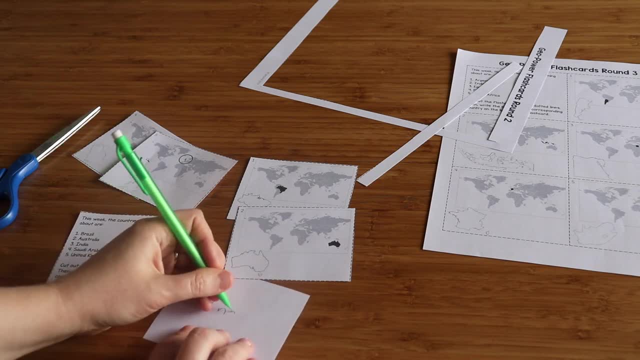 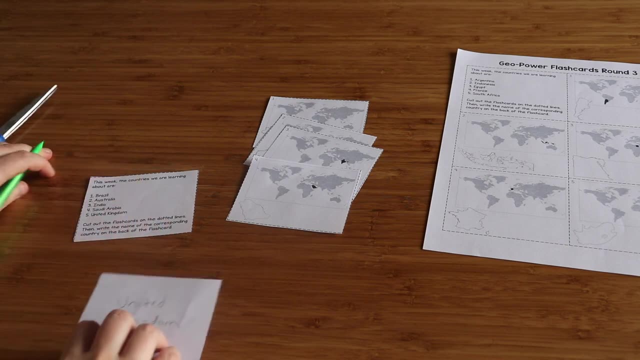 of that particular place as well or connect it to something they might already know. Also, all of the GeoPower systems that I have set up starts with some easier, larger countries first and then works its way through to a bit more difficult locations. as the program goes on, You can. 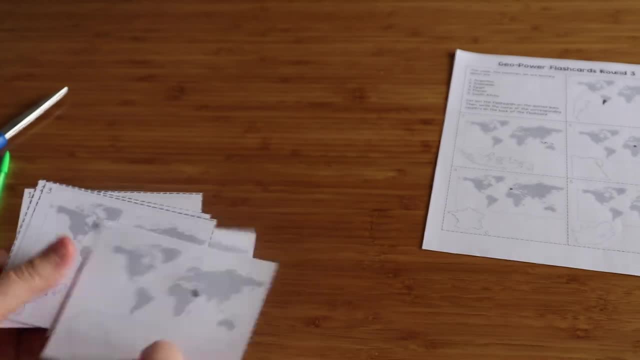 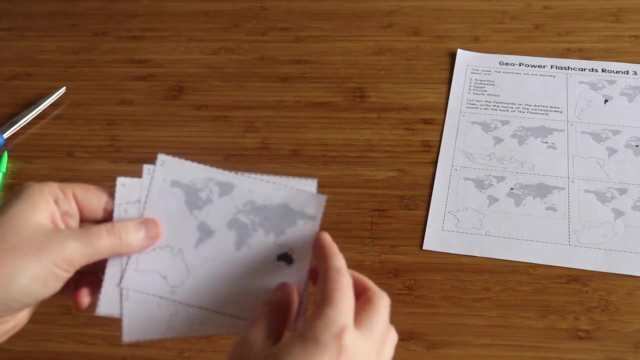 actually follow along in a free sample I have put together for you. that's also linked below, So students are preparing the flash cards. While this is happening, you pull up the review slideshow that corresponds with each round of the program, which has the same countries that are on their. 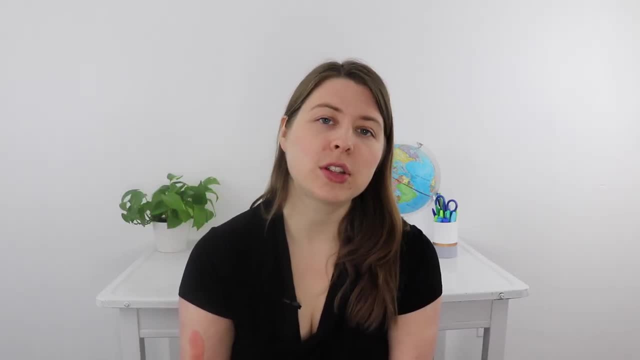 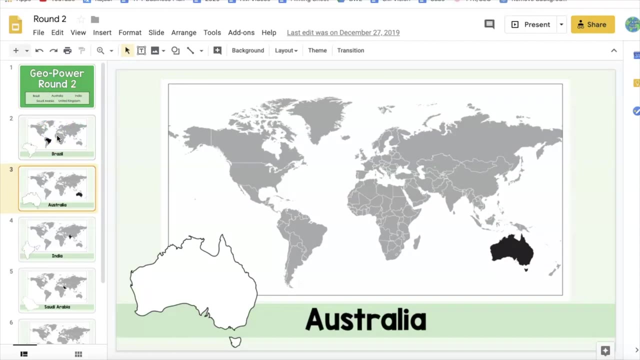 flashcards in a slideshow format. This allows students to see it bigger on the screen and allows you to use the slideshow to go over it and discuss them. Then the last slideshow of each round has a blank map, which is perfect for students to practice the countries of that round as well as. 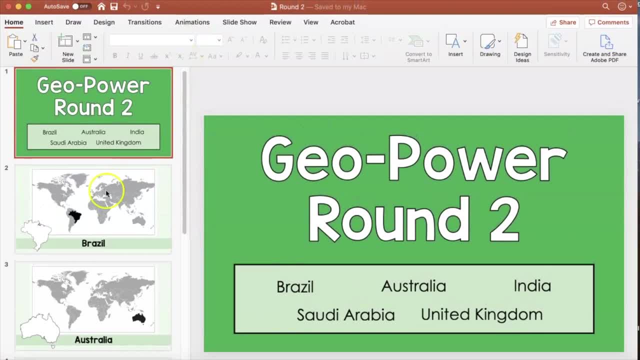 countries that they want to see. So if you want to see the countries that you want to see, you can go ahead and click on that and you can see the countries from any previous rounds, and there's a lot of fun review games that you can do with that. One of my favorite to do was board races, where I 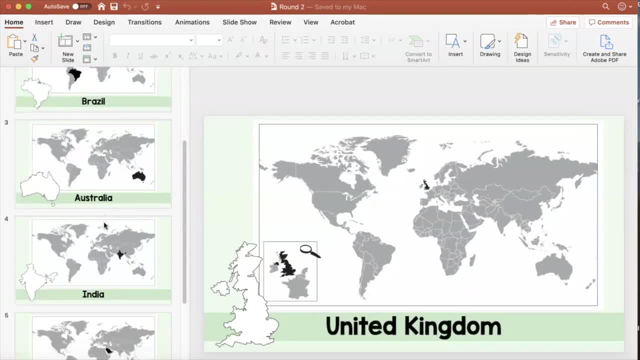 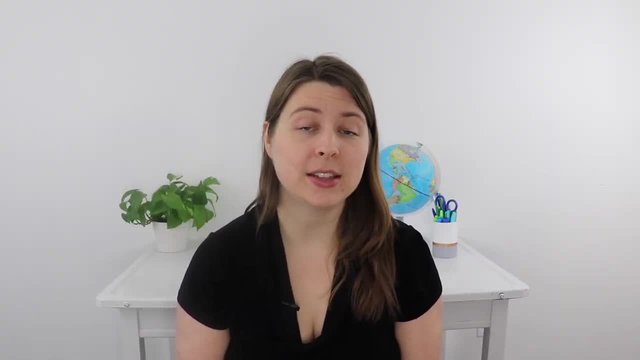 divided my students up into two or three teams and it was a race to see who could find that country first. Then, at the end of that round- which for me I typically did one round over the course of two weeks- I would review it a few times during the weeks, maybe two or three times, just for quick. 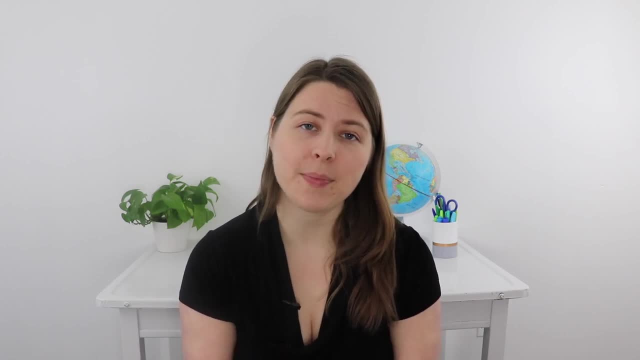 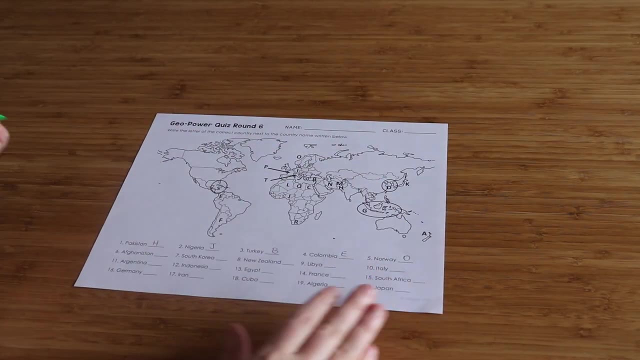 five to ten minute reviews, just so it didn't take up a lot of time. Then there would be a short quiz at the end of that round that students would take and that would just assess to make sure they knew where those countries were As the program continued. they 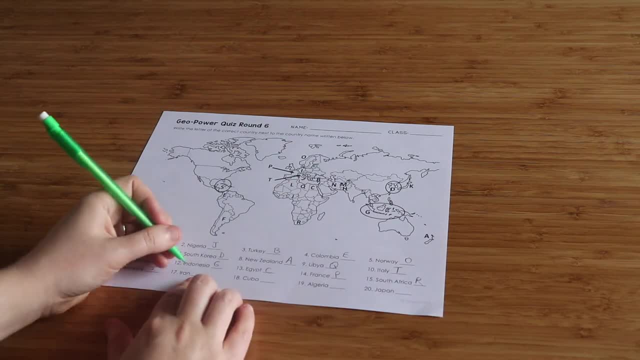 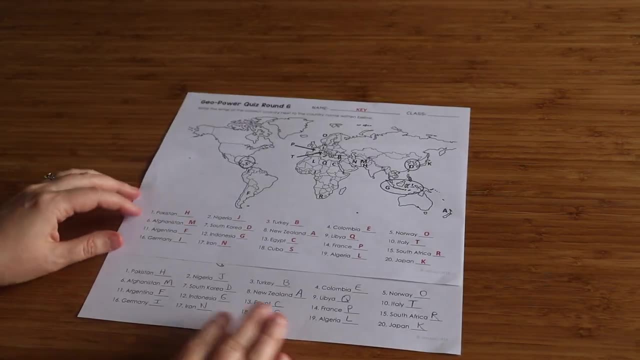 would be held accountable for up to three past rounds of GeoPower, so up to 20 countries, And this was a chance to make sure it wasn't. let me learn this and forget it situation. we were continuing to practice it. Of course, when the program's done, there is a final test as well. but it's not something the students were really nervous about, because you know there's a lot of people out there that are really nervous about what's going to happen in the future. So if you're really nervous about what's going to happen in the future, you're not going to be able to do it. 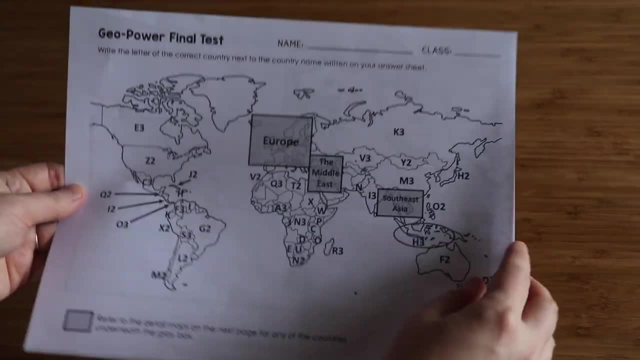 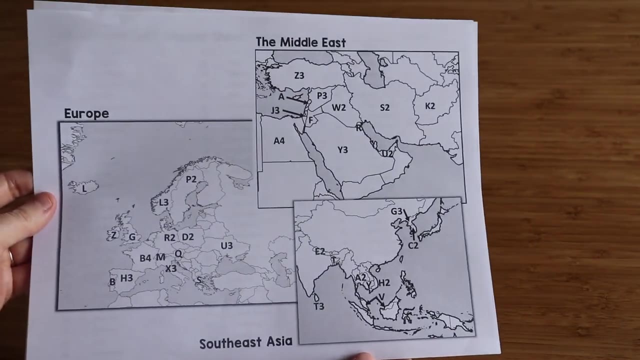 So I think it's a good idea to do this, because we had continued building and reviewing these the whole time, And one of my favorite review games for these quizzes or tests would be to do time trials with my different classes and see how quickly they could actually go through where. 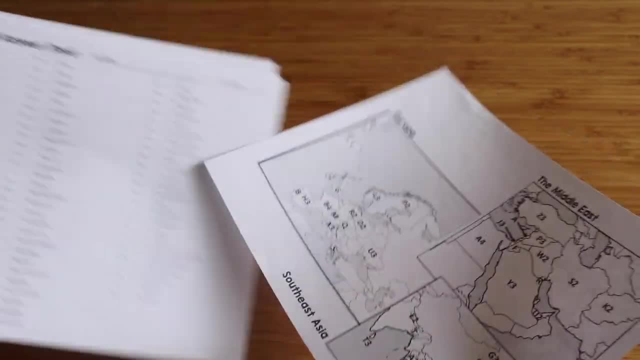 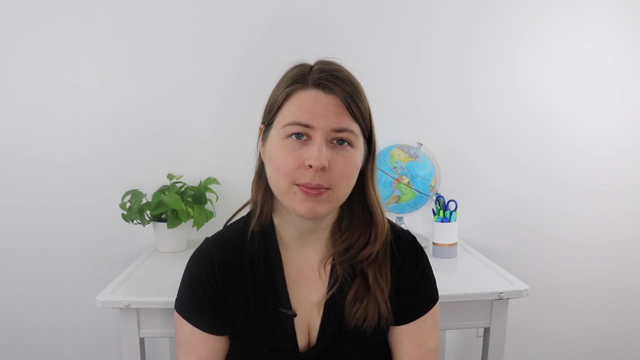 the locations of the countries are. Now. sure, some critics might say, with all the maps and mapping tools available online, do students really need to know where countries are? But I would actually say the same thing about math facts, With calculators everywhere, including on our phones. 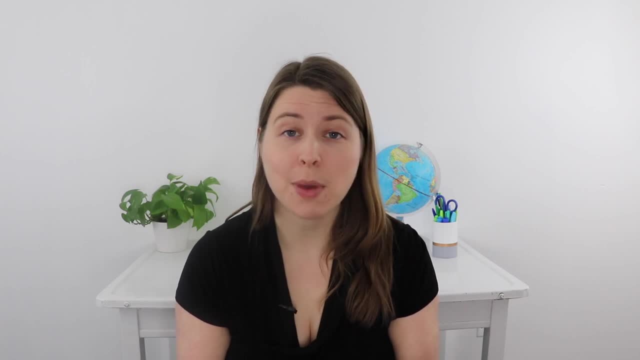 do they really need to have their multiplication tables memorized? I think yes. Having some of these base pieces of information memorized can be helpful in a lot of ways. One of the best ways is with current events. When students have this baseline of geography, it's a lot easier for them. 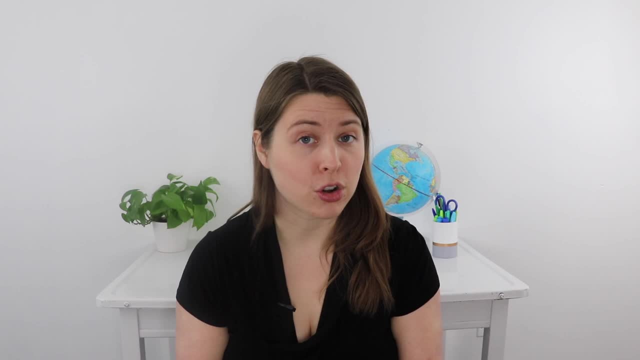 to know where something is when it's happening, because they either know where that country is. or, if they don't know where the country is, you can give them a context clue and say, oh, that's right by this country that we studied, And then it helps them have a little bit more context. 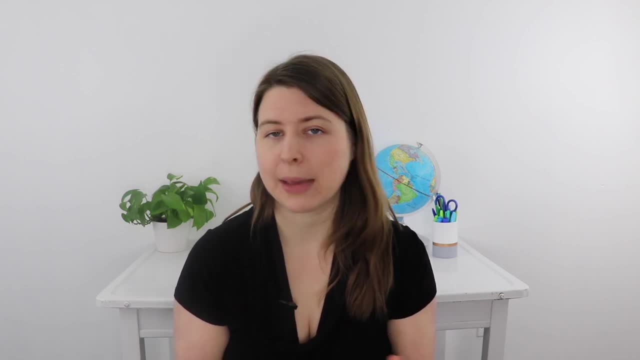 Originally I used this as a full year program, which is like my main GeoPower program, which consists of 16 rounds, 80 countries total. However, if someone's looking for a smaller commitment and maybe wants to start their year off with some geography skills, I also put together six round. 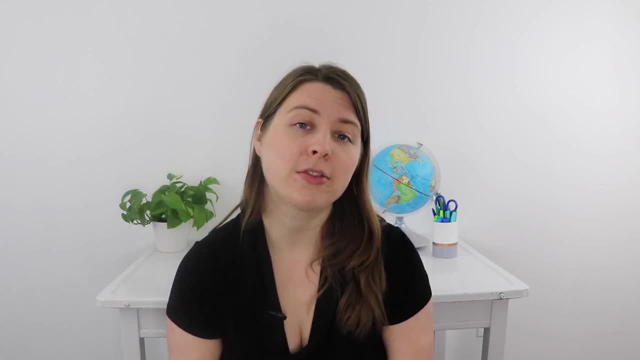 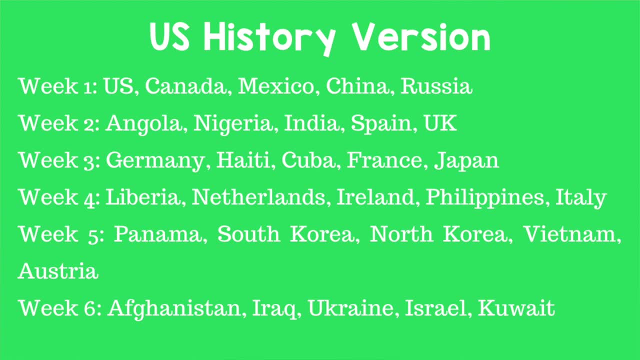 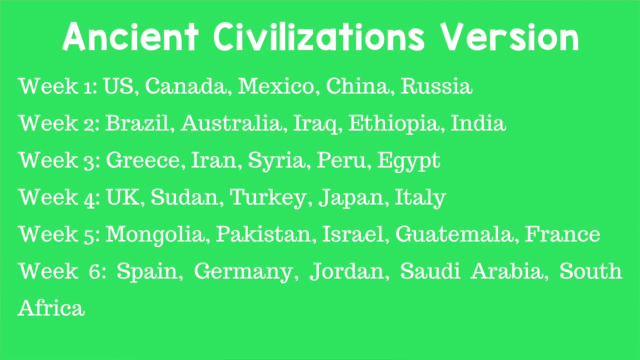 easy to use and they're really easy to use and they're really easy to use. These versions are great because it gives you the chance to really personalize these 30 countries in each set to the places that students will be learning about either in US history or ancient civilizations. 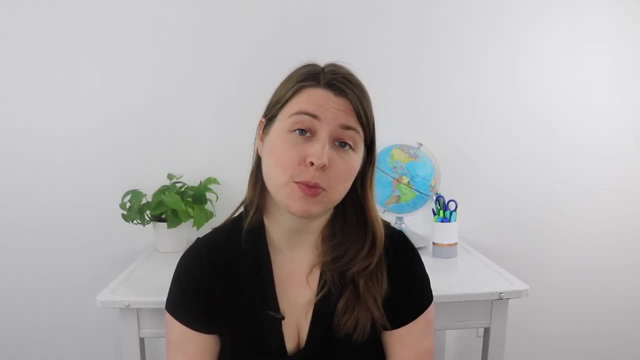 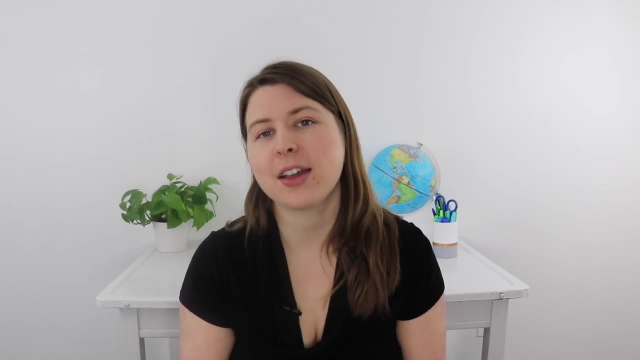 And while I don't think this affects many of you, I do have a Spanish-speaking country version as well- which is a four round program with 20 countries- the 20 Spanish-speaking countries outside the United States, As I mentioned earlier in the video. 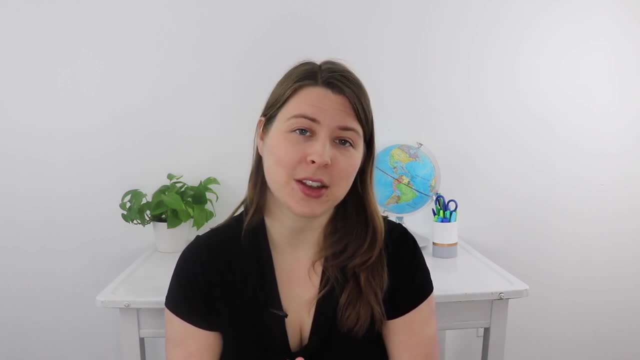 for the next two weeks, I am putting all of these resources at 20% off, and if you want to actually try this for yourself, you can get round one of the GeoPower program for free with the free sample link in the description field of this video.